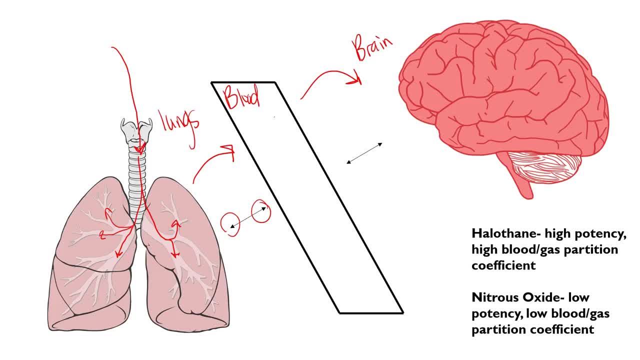 the solubility and the permeability of the membrane and whatnot. So this brings us to two important definitions to know. Potency is the first one. Remember, potency is basically a measure of it's how it's basically the lowest dose of a drug needed to begin to show its effects for that drug. 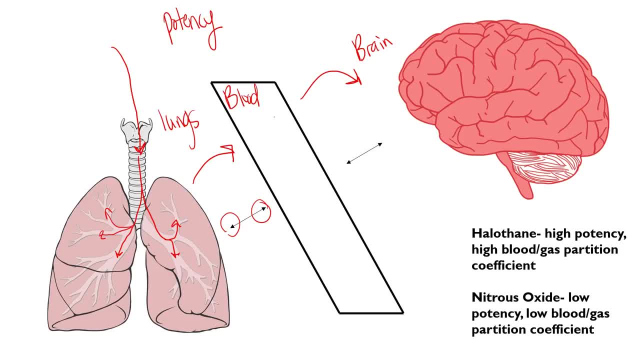 the minimum effects of that drug. For example, you have drug X. let's say you have a drug X and drug Y And drug X at 20 milligrams. that's the first point at 20.. So you say you're slowly raising the dose of the drug. And finally, 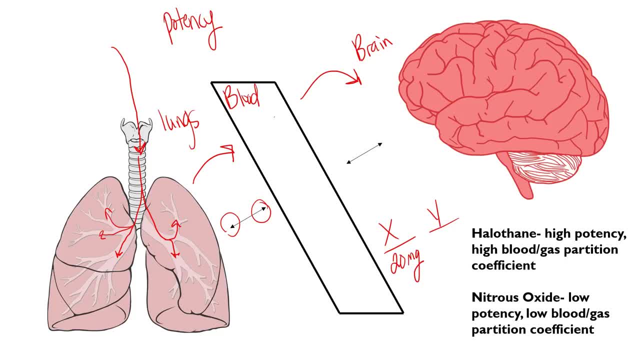 at 20 milligrams that you give the patient, they begin to show the effects that, whatever the effects that drug X is, whether it be vasoconstriction or an increase in blood pressure or whatever the drug does, 20 milligrams would then be basically the point at which the potency of the drug is marked. 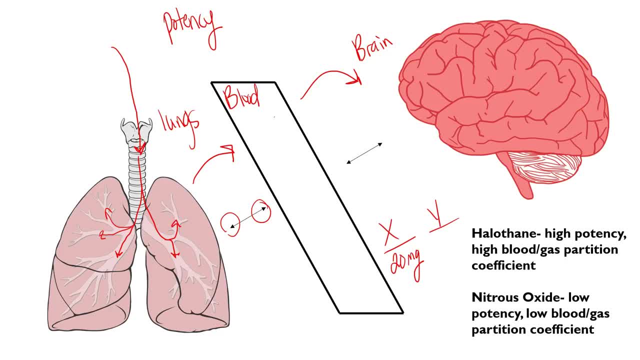 out like, let's say on a graph: Whereas drug Y, drug Y, so let's say it's a single dose of a drug, a similar class of drug. it only starts showing its effects at 40 milligrams. So basically, potency. that's how potency works. So a drug that has an increased potency, it just means that the drug will show its effects at a lower dose. So X here is the one that has the increased potency compared to Y. Now, what affects potency? The main thing that affects potency as far as our concept that we need to know. 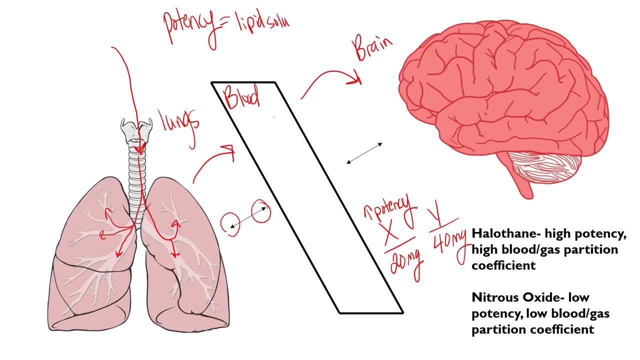 is going to be lipid solubility Solubility. An increased potency occurs when you have an increase in lipid solubility. Well, of course that makes sense. The cell membrane is a phospholipid bilayer And this is a lipid soluble membrane. So drugs that are more lipid soluble can more easily cross. 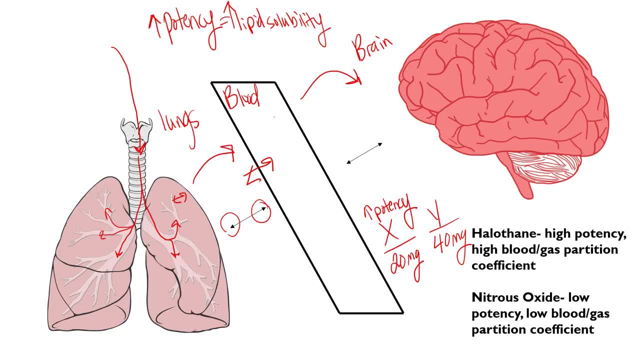 over these bilayers. See, like in the lung, the alveoli, they have a lipid bilayer in one of its many layers. It has to go through, but there's a lipid bilayer in there somewhere. Then, even like going into a blood vessel, you're going to have 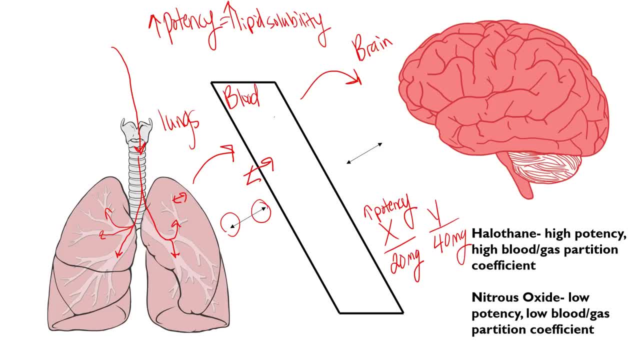 to pat the cells, the endothelium, you know the endothelial cells of a blood vessel that has a lipid bilayer for those cells. Again, going into the tissues, we know that tissues are just a group of cells And obviously 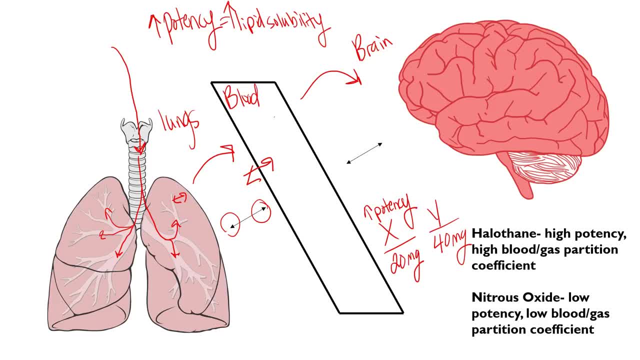 those have lipid bilayers. So that's all dealing with potency. So let's not confuse potency with the next thing that we're going to talk about. This is blood solubility. Now we said that an increase in potency will just mean that. 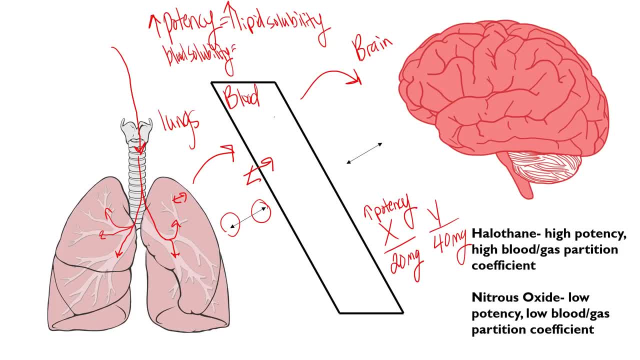 you need less of the drug or, I'm sorry- it will show its effects at a lower dose, Whereas a decrease in blood solubility means that the drug will act faster. It doesn't matter what the dose is. So now we're not talking about the 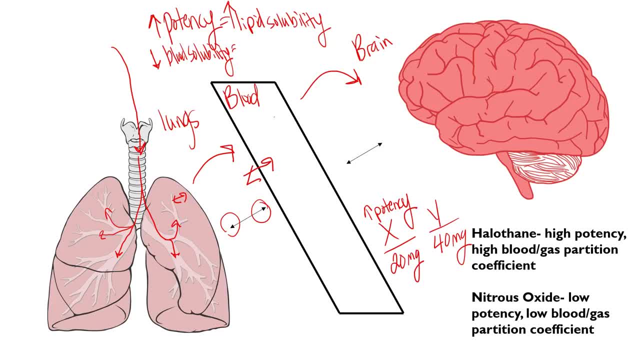 dose. It doesn't matter what dose it is. From the time you give the drug- let's say you give the drug- a blood drug- at time, zero, zero minutes, And after one minute the drug, you know the drug- begins to show its effects. 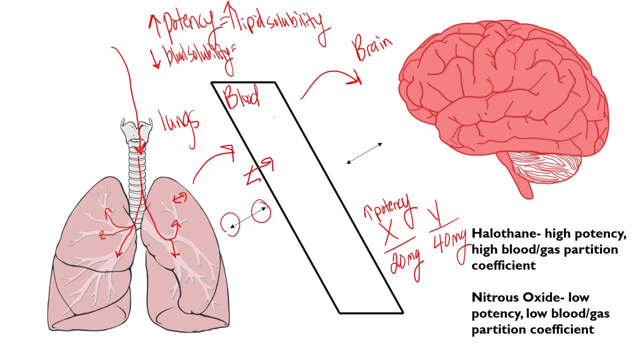 which means it's reached the brain all the way to the brain and it's now in the brain having its effects. So a drug with a lower blood blood solubility just means that you will have the effect. the onset of action of the drug onset. 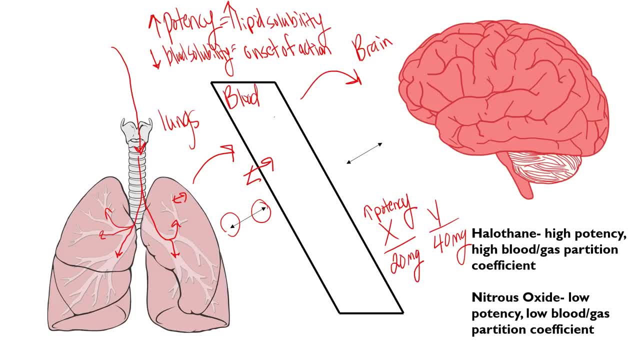 of action will be at a lower time. increased onset of action, basically, So it doesn't take as long, And ways that some things that we they'll try to do. basically to kind of compare these two, There's other terms within these two. So for blood solubility they use something called blood gas partition coefficient. 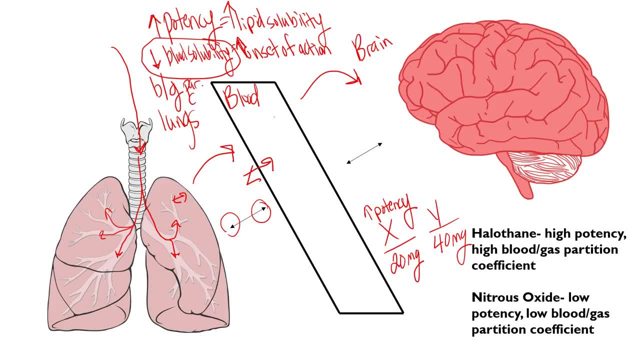 I'm just going to put blood gas partition coefficient. That's just saying it's comparing the blood solubility of the drug over the gas solubility of the drug. So if you have a decreased blood solubility for whatever drug, let's say drug x. 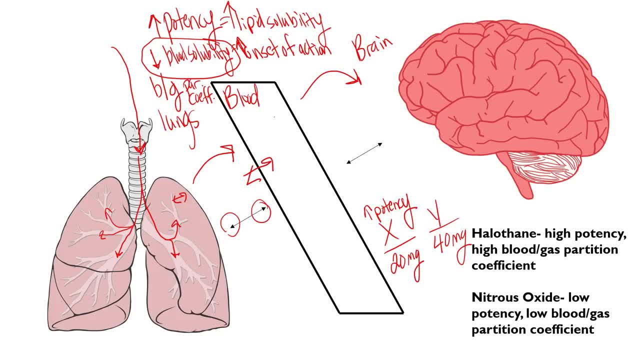 if you have a decreased blood solubility, imagine that this is a fraction. that just means you have a decreased. the top number here, the b or the letter, I'm sorry- is going to be lower than the bottom number, the gas solubility of the drug. So that means 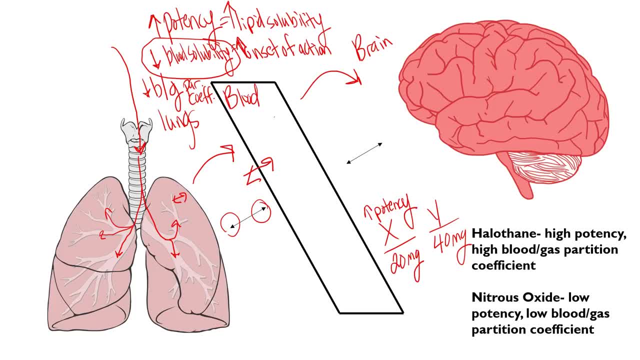 that this will be as low. So a decreased blood solubility equals a lower blood blood solubility here, And that's just a- a decreased blood gas partition coefficient. and they may not always tell you blood solubility. they may give you a blood gas partition coefficient. it'll be some decimal, or could. 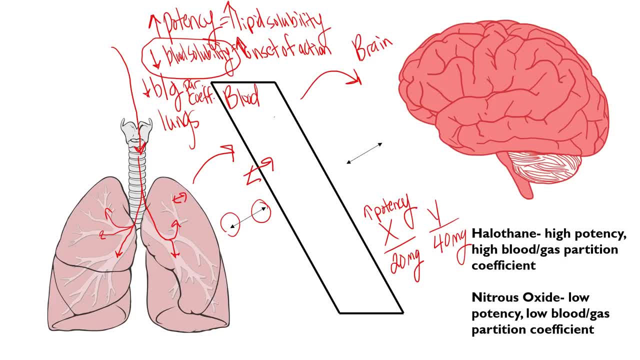 even be a whole number, to some decimal or whatever, and so that's a way that they're going to tell you what the blood solubility is by giving you this blood gas partition coefficient. a way that they can tell you the potency is to either describe the lipid solubility to you, if 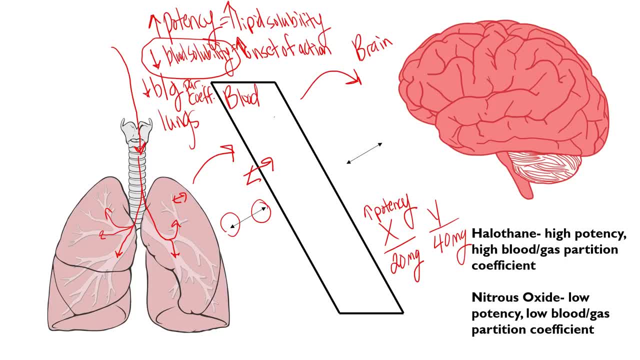 there's an increased lipid solubility. we know there's an increased potency, or potency affects, like we know that lipid solubility affects potency. another thing that potency will affect is the minimum alveolar concentration, that is- and really i just like to write 50, it's not usually. 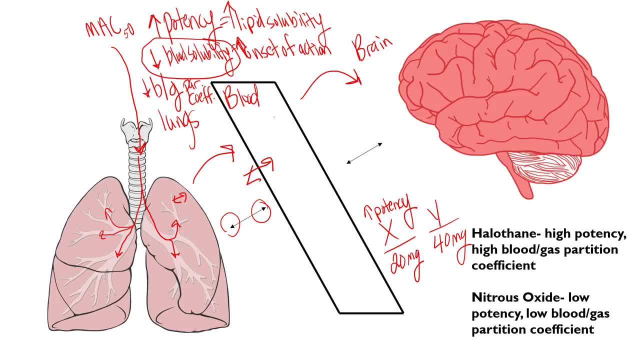 written that way, but it's in the definition. you understand why the minimum alveolar concentration of a drug is the lowest amount of the drug needed in the alveoli to begin to show its effect. So that's very similar to potency, But in this situation it's the minimum alveolar concentration needed to show the effects of an. 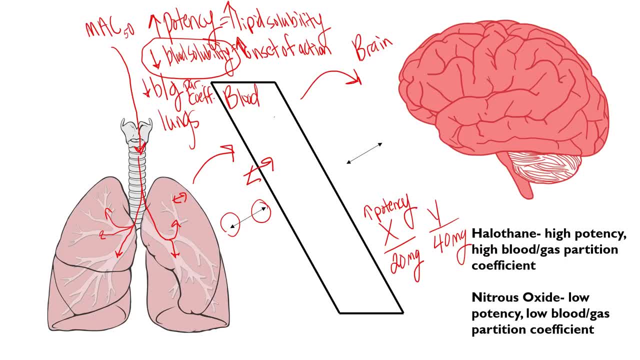 anesthetic in 50% of the patients that are reported, Let's say in a trial of 2,000, when 1,000, right at the point, right at the minimum alveolar concentration, as you're increasing the concentration of the drug given to all those 2,000 patients, when 1,000 patients. 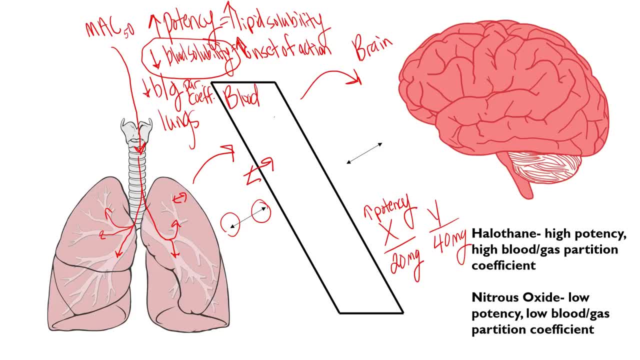 which would be half of the total population, begins to show its effects. whatever that lowest dose was, they start to show the effects is the minimum alveolar concentration And I just wrote, like I said, it's not usually written MAC50, but you can write it as that. So an increased potency. 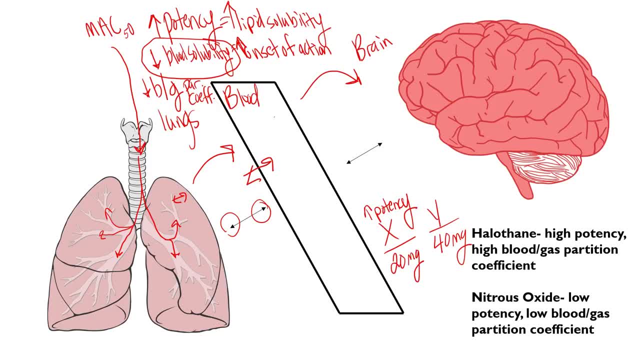 means there's an increased lipid solubility and means there's a decreased minimum alveolar concentration. Because, think about it, if you're starting to show the effects and all the people in your trial, or 50% of the people in your trial- at a lower concentration of 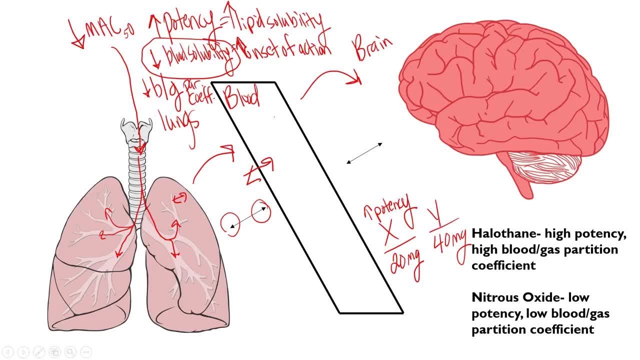 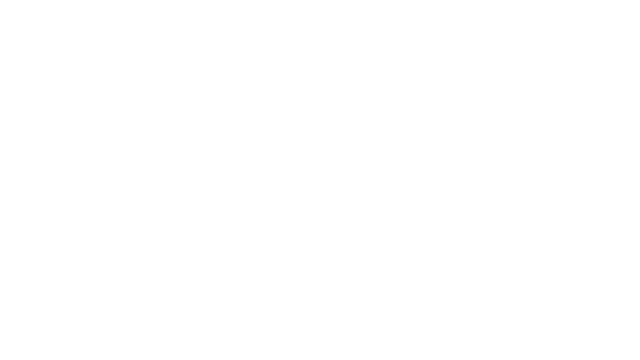 a drug. that is the very definition of potency. That means you have an increased potency. So see, this is opposite here. so be careful of that: Increased potency means you have a decreased MAC50.. So now let's get kind of into, let's get into the actual what I want to talk about. 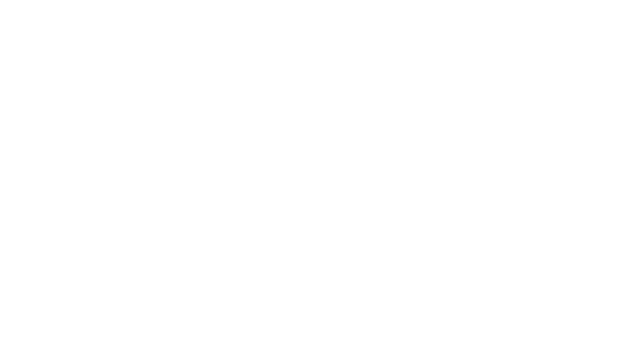 You have a drug. this is the second gas effect and I'm just going to take two of the inhaled anesthetics: Halothane. there's other ones, but I'm going to. this is simplified Halothane and nitrous oxide. Now, basically, the drug is taken. 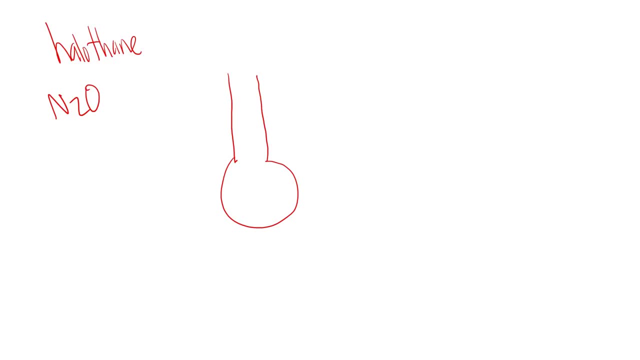 you know, it's inhaled through a ventilator and taken down into the alveoli. Two some things you need to know about these two drugs. just comparing these two. Nitrous oxide has a very low blood gas partition coefficient. What does that mean? That just simply means it has a low blood solubility. 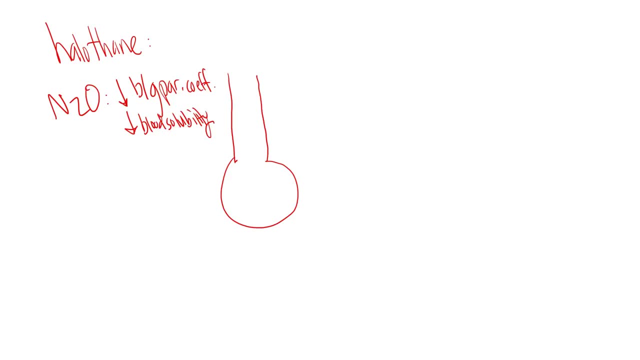 So imagine you give nitrous oxide by itself. Let's just first say you give nitrous oxide by itself. You give the nitrous oxide by itself and it's mixed with some oxygen. So let's say we have- I don't know, 70% is nitrous oxide and 30% is oxygen. okay, Is oxygen. So this 70% nitrous oxide? 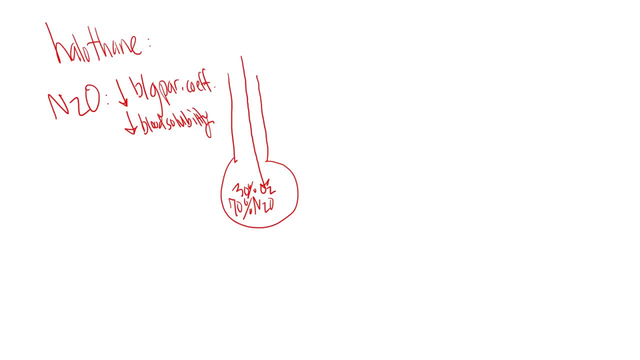 because it has such a low blood solubility. it has a very low blood gas partition coefficient, low blood solubility. we know that it will show its effects very rapidly from the time it's given. the reason is because here's the blood vessel and here's the brain that we saw earlier and 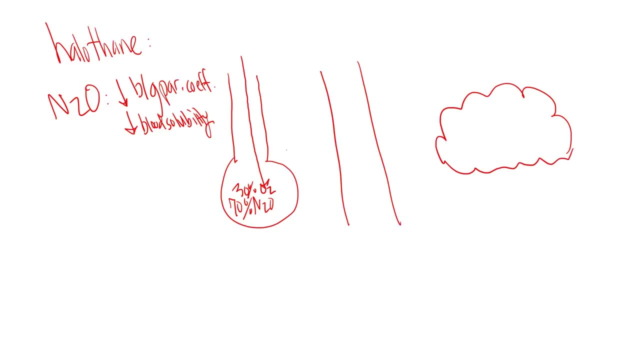 sorry for the drawing. here's the brain and here's so. we know that it goes from the lungs to the blood vessels, to the brain, and then it can also go back, but it has to be in that order. so nitrous oxide, when it does end up crossing over into the bloodstream, it's, it's has such a. 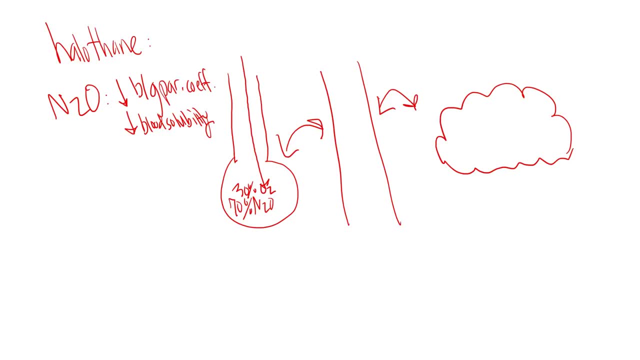 low solubility in blood, that it doesn't stick around in the blood very long and because and so because of that it tends to go. it tends to jump quickly from the lungs to the blood and easily gets over here to the brain. and it happens very easily because the blood solubility doesn't hold. 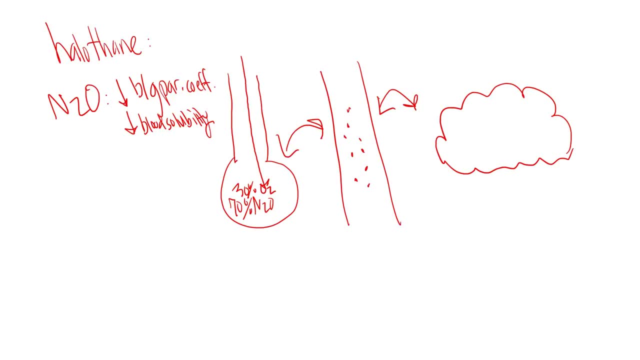 it in the blood, whereas halothane has a very high blood solubility, blood solubility that has a high blood solubility, that has a high blood solubility, that has a high blood solubility, high blood gas partition coefficient. so when halothane comes down, it enters, when it does. 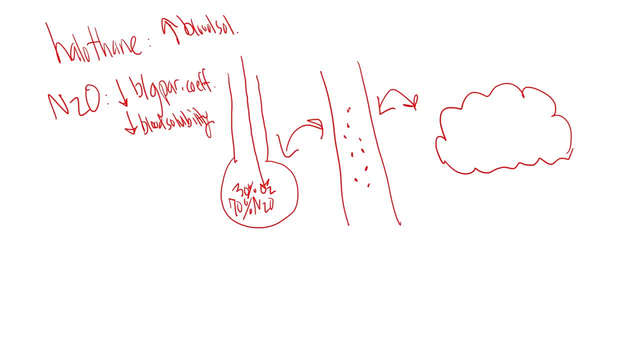 enter into the bloodstream. it has a very high blood solubility, so it tends to just hang around in the blood and you have a trouble getting it to the brain as fast as the nitrous oxide can get. so in essence, what that means is that nitrous oxide can equilibrate, because you know how the 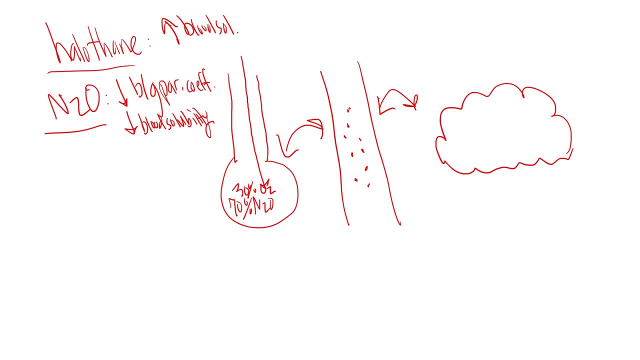 you know how concentrations work. basically, if you have a box and it has two sections, and this was a permeable, semi-permeable membrane, and let's say, halothane is here or whatever, just a substance that can go to either compartment, this can travel back and forth. if you put it all, 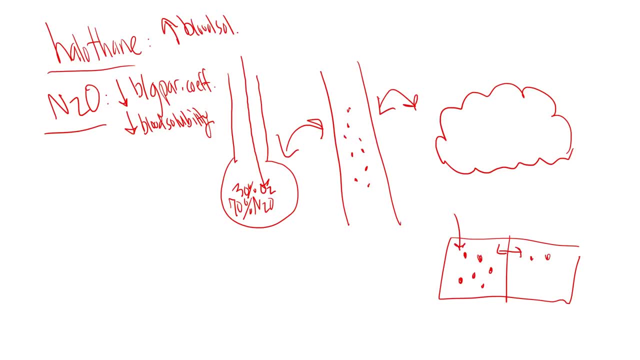 if you put all this in here, eventually the amounts will equal out, right, eventually it'll basically equal out and it will basically you eventually equilibrate, and that's what's happening. but but nitrous oxide can equilibrate faster and that's the reason that nitrous oxide has that lower blood solubility, thus the lower blood gas. 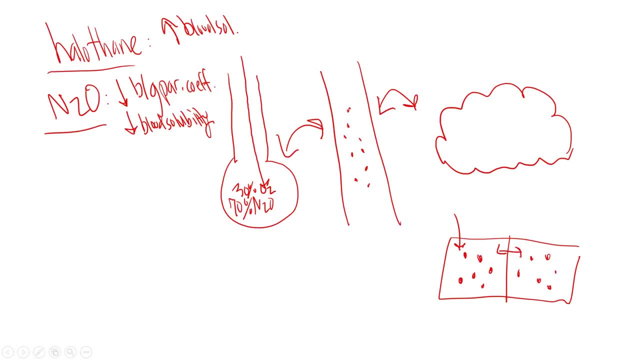 partition coefficient, whereas halothane has a higher blood solubility and thus a higher blood gas partition coefficient. now the potency: it's completely different. we said that nitrous oxide acts fast because of this low blood solubility, but the potency is very low for nitrous oxide. 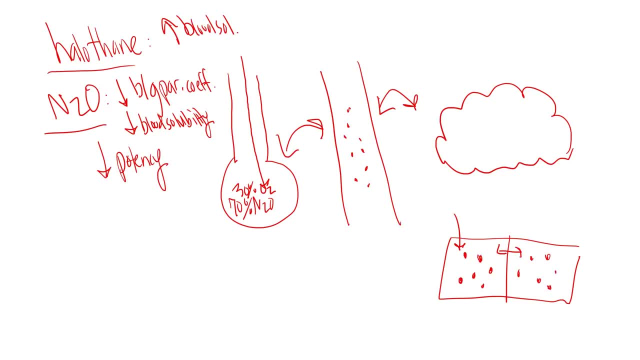 this means that you need a large amount of nitrous oxide before you would ever see the effects. and remember earlier i said that potency is primarily based off of lipid solubility. we have a low potency because the lipid solubility is very low for nitrous oxide. okay, so 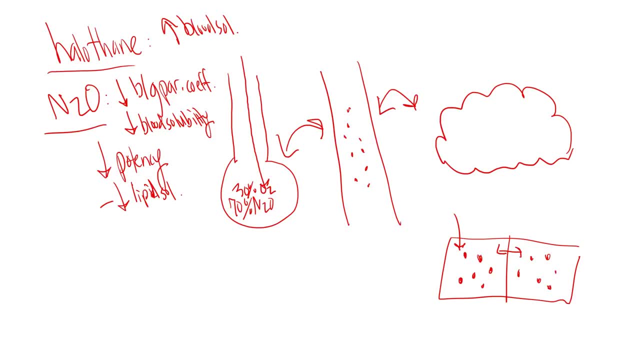 you. that's so. that tells you you're going to need a lot of nitrous oxide to show any effects, and this makes sense as to why nitrous oxide is rarely ever given as just one drug, like, say, to act as an inhaled anesthetic. you always usually see nitrous oxide giving given with another inhaled anesthetic. 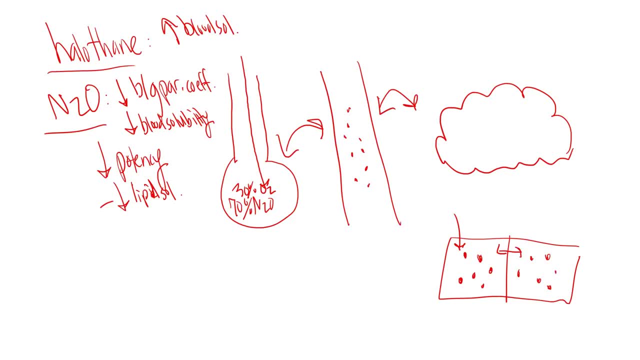 and inhale another inhaled anesthetic that would maybe need help equilibrating. so it's going to use nitrous oxides- a fantastic ability of decreased blood solubility that has a rapid onset- and it's going to. basically, nitrous oxide will assist halothane to equilibrate faster and halothane is going to help nitrous oxide. 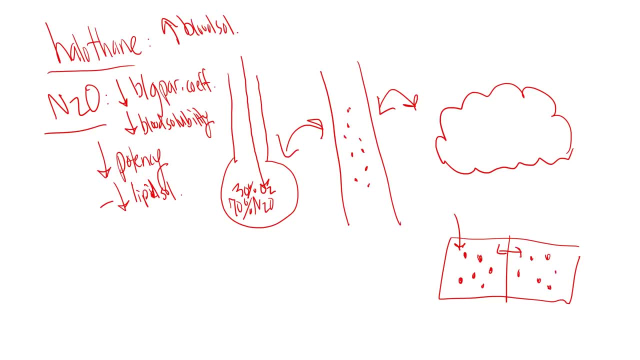 by not needing as much of a dose. so you can give a very low dose of halothane and still see the effect. so they're helping each other. so that means halothane. halothane has a high potency and remember, a high potency means a high lipid solubility. right, it can. it can cross over the membranes extremely fast. 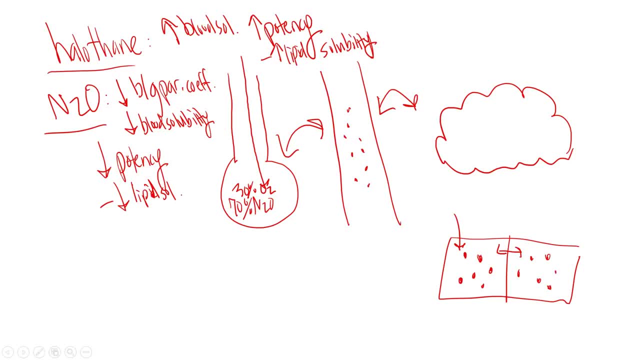 so that's dealing. so don't don't mix it up. and increased lipid solubility means you have an increase in. i'm sorry, you don't need as much of the drug before you see the first effect. this has nothing to do with the, the speed, the potency has nothing. 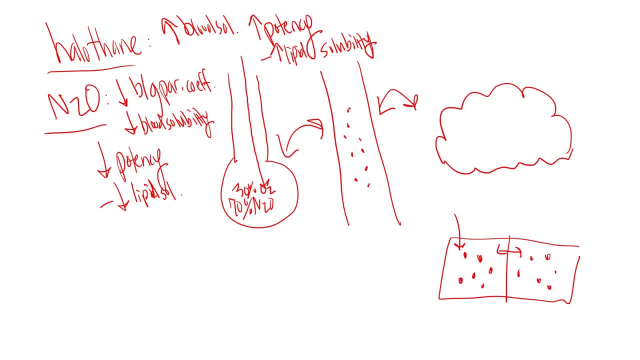 to do with the speed of of onset. that is all determined by a blood solubility and you need a low blood solubility so that it doesn't get trapped in the blood. that kind of the bloodstream of the body and it's able to get into the tissues faster and equilibrate, like nitrous oxide, is now. 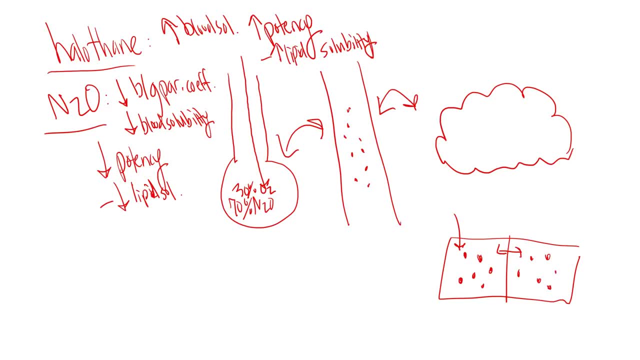 let me show you why giving nitrous oxide with halothane makes basically makes the drug more effective. basically it has to deal with concentrations. so I'm gonna draw another alveoli. let's let. now. let's give nitrous oxide and halothane together. 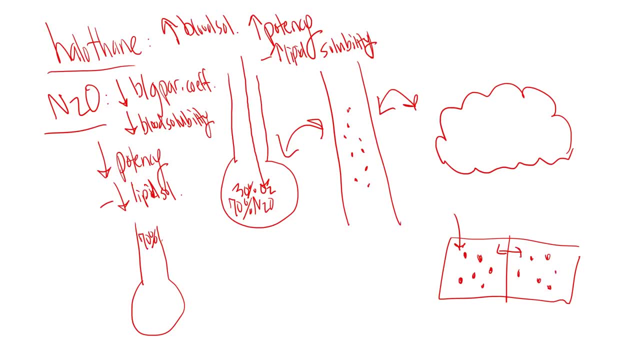 and naturally with oxygen. let's say we're gonna give 70% nitrous oxide, 28% oxygen and 2% halothane. those ratios should make sense for at least in our example, because I said halothane has such a high potency that you would see the effects at a lower concentration. it makes sense. 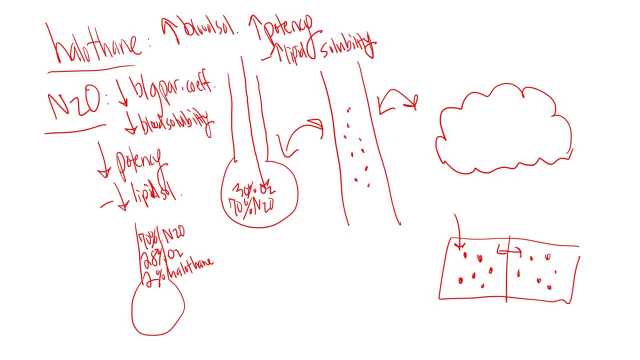 that you need a lot of nitrous oxide because the potency is very low, and then obviously oxygen has to be at a lower concentration, and then obviously oxygen has to be at a lower concentration and then always be with it. now here's why it's this works. you give these three together. remember I said 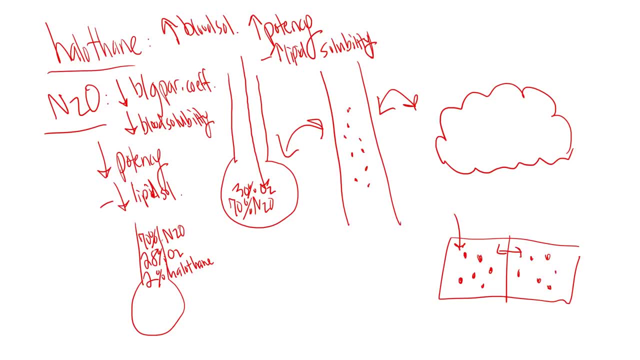 nitrous oxide has its effects that happen extremely fast and it's because, when you get these three- the first one to equilibrate among all three of these things- the alveoli, the blood and the brain- the first one to equilibrate is nitrous oxide. so what does? 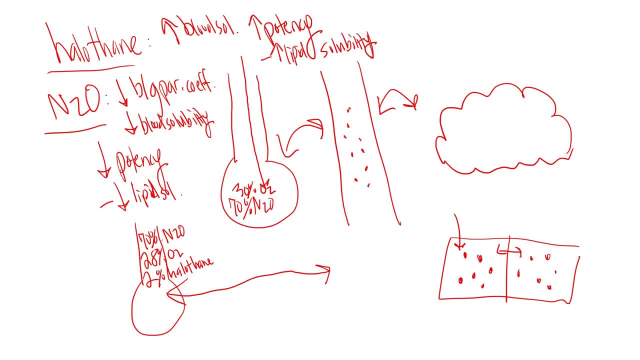 that mean well before oxygen and halothane ever get a chance to equilibrate between the three compartments, nitrous oxide has already done so. so imagine we give these three. nitrous oxide will equilibrate between- let's just ignore the brain right now. nitrous oxide will equilibrate between 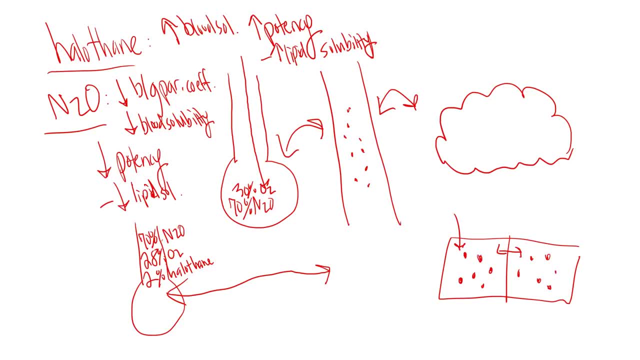 the alveoli and the blood and the blood vessels, and it will basically, you know, be equal on both sides. so let's say it'll become 35% and 35%, right, half of 70, 35 and 35, and it will happen, it will equilibrate way before. 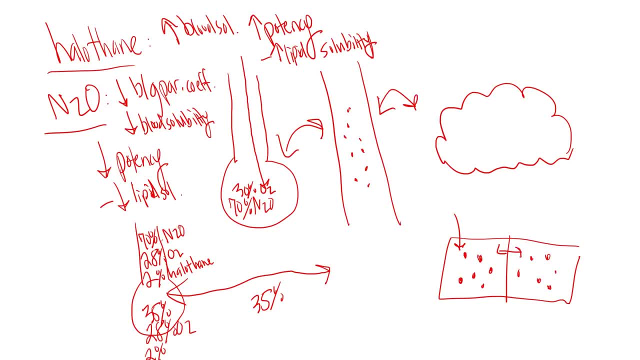 the oxygen and the halothane have even had a chance to, and that's because of that blood solubility the blood solubility is so low. so in essence, now let's look at the comparison. here's a. so you take these three, you add them up, that's a hundred percent of the gas, right? total. 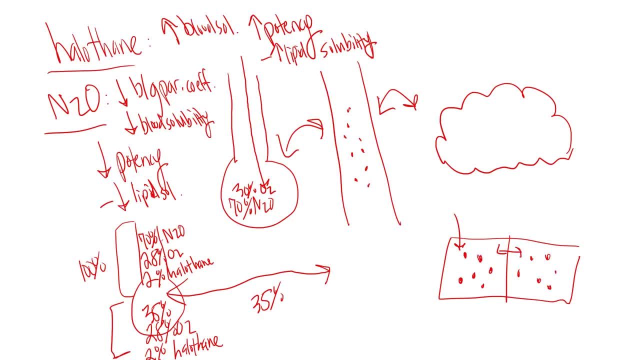 that's entering in now. look now when you add these three up, because half of the nitrous oxide has already. it has already left to the blood vessels and it's already been equilibrated. if we're ignoring the brain tissue, that means that now the new total is 35 plus 28 plus 2. so in other words, the new total is at a lower percentage. this is a lower percentage here. so now, as far as the concentration is concerned, we didn't change the levels of oxygen. we didn't change the levels of halothane or even change the levels. the only level percentage that changed in the alveoli itself was the nitrous oxide. so now the 28% oxygen is now at a lower percentage here. so if we look at the 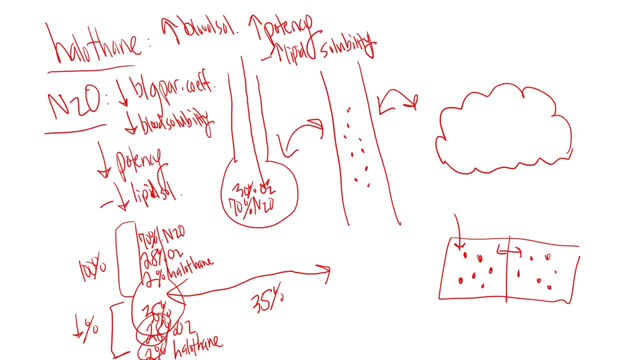 and the 2% halothane. there's far more of that as far as concentration wise, because all of that 30, the other 35% of the nitrous oxide has left over to the blood, So now you have a higher concentration. 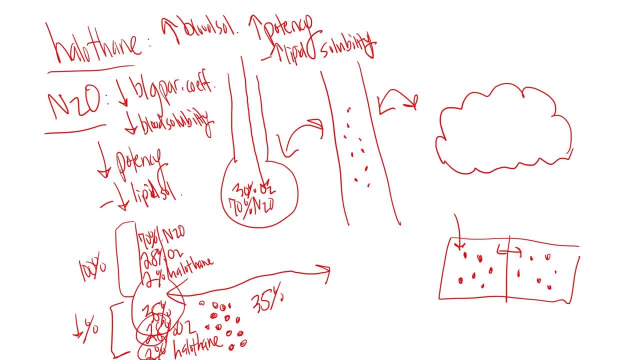 of halothane and oxygen in the alveoli and thus you will have a stronger effect of that halothane. So whereas before we started out with you know 2% halothane, now the halothane percentage is actually gone up in relativity to relative to the other two because the nitrous oxide 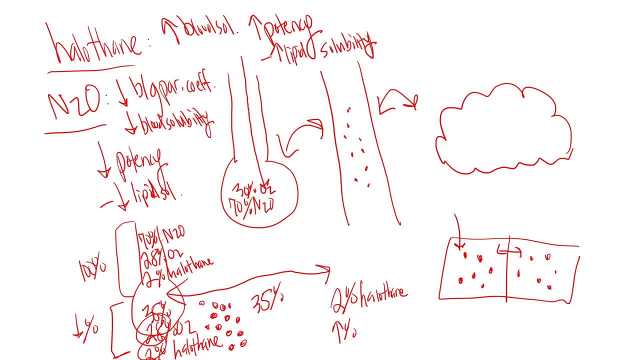 which was the primary gas coming in from the ventilation machine, has been cut in half. So now, therefore, they're a lot closer to the number of the nitrous oxide. now. So the concentration as far as the percentage, even though we haven't put any more halothane in the percentage of halothane. the percentage of halothane that we put in the alveoli. the percentage of halothane that we put in the alveoli. the percentage of halothane that we put in the alveoli. the percentage of. 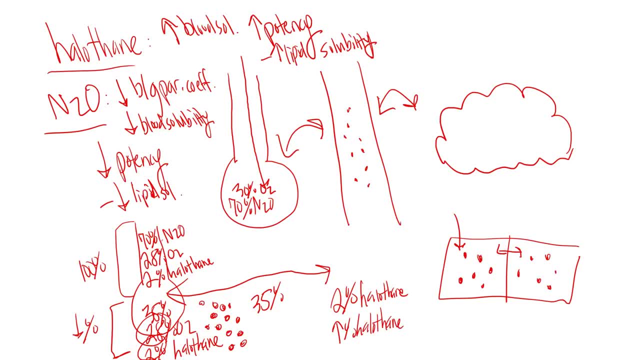 halothane has gone up And the percentage of oxygen has gone up. That's what's called the second gas effect, And that's how we get a stronger effect of other anesthetics using nitrous oxide. Now, what is diffusion hypoxia? It's just completely flip it. 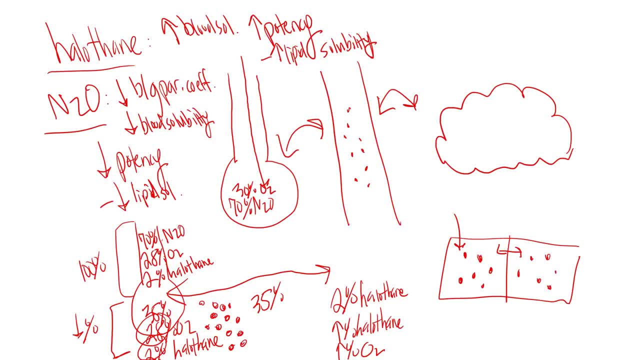 Imagine we turn the ventilation machine off. When we turn the ventilation machine off, here's up here and here's the bloodstream. Remember that the nitrous oxide has a equilibrated Now everything has eventually equilibrated, but we had a stronger effect. 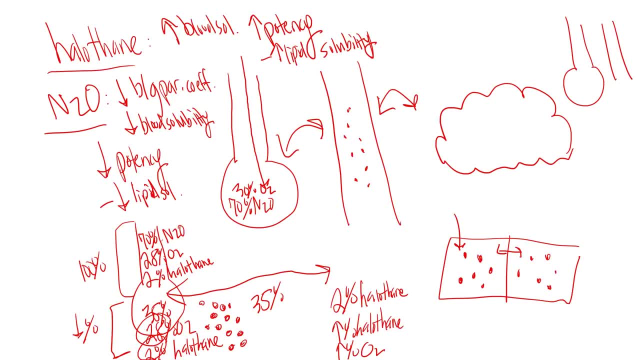 because the nitrous oxide equilibrated far faster, So it will help with showing the effects better And basically it will help to equilibrate with these other ones because we're messing with the concentration gradient. What happens when you turn the machine off and 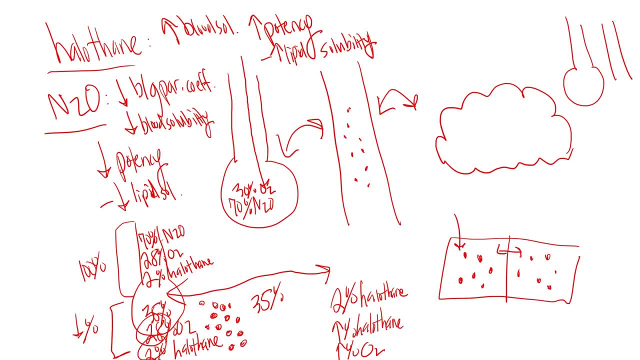 the patient needs to recover. Well, all of that, the concentration of the halothane, I'm sorry, of the nitrous oxide, that large percentage of the nitrous oxide that it, equilibrated between the three compartments, now needs, is going to begin to rush back, because it's 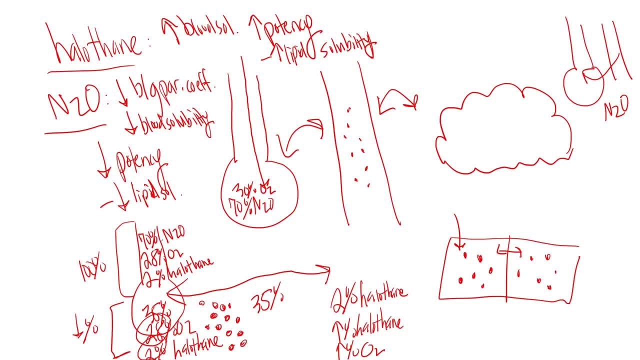 being cleared from the body right, And it's being cleared through the lungs. You're breathing it out, So it all rushes back. And I said that nitrous oxide has such a low blood solubility that when it's coming from the tissues, like the brain, like muscle and everything else, when it's coming from 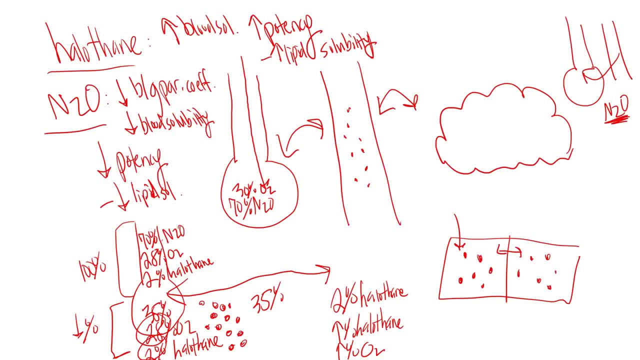 those tissues and it's going to the bloodstream to get to the back to the lungs. the problem is it can't. it can't be. It's not soluble in blood. It has a terrible blood solubility, So it basically rockets in. 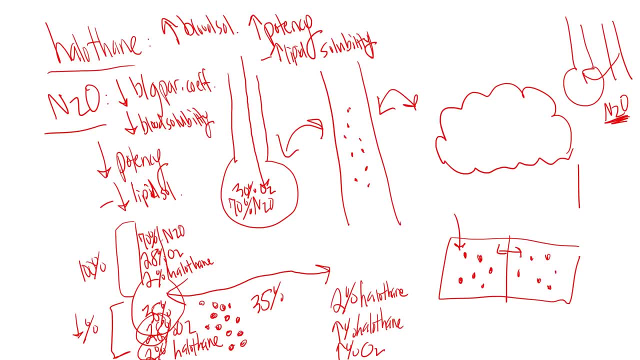 speed over to the alveoli, And it happens so fast. The concentration of nitrous oxide rushes to the alveoli so high that now remember before the concentration of oxygen had actually been increased when nitrous oxide rushed to the bloodstream, but now it's the